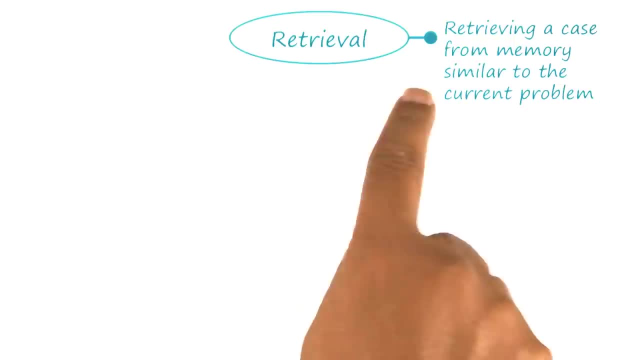 case-based reasoning consists of four steps. The first step is retrieval, and we already considered this when we were considering learning by recording cases. K nearest neighbor is one way of retrieving cases. This is from memory. Once we have retrieved a case from memory, that is. 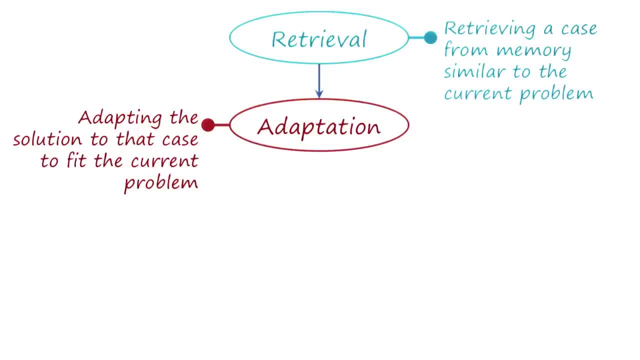 relevant to the current problem, we need to adapt it. For example, in the previous problem we had the d case and the q problem and we needed to adapt the d case into the q problem. There are many similar examples. All of us program. 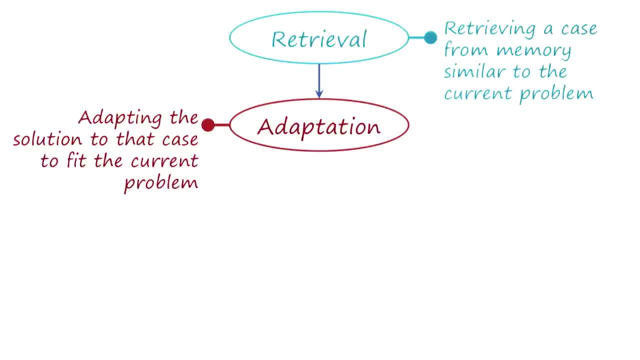 and all of us, as computer programmers, sometimes use case-based reasoning. We are given a new problem to address and we often look at the design of a program that we have come across earlier. So that's retrieving a case and adapting that particular design of the old program to solve the new problem. 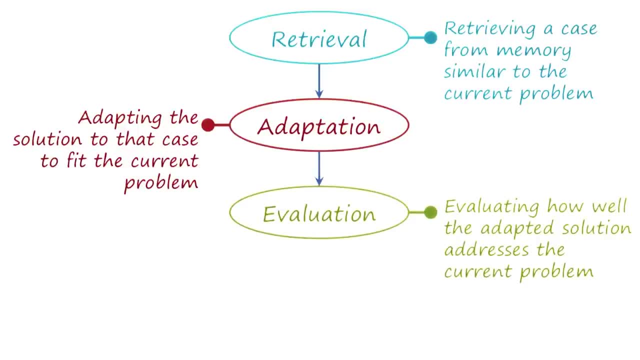 Once we have adapted a case to meet the requirements of the new problem, we have a candidate solution for the new problem. But that candidate solution needs to be evaluated, For example in the navigation problem. when we have a solution to the q problem, we can evaluate it. 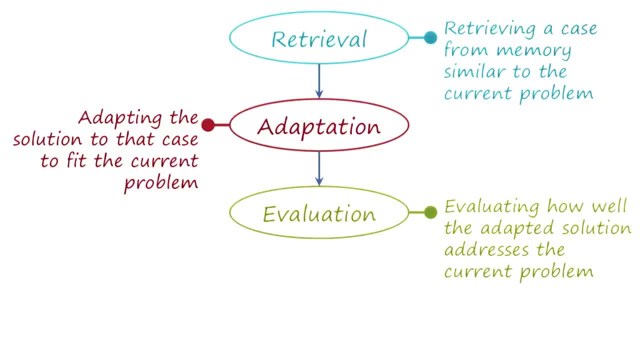 but it will actually take us to the end location. We can do a simulation, we can walk through it. As we walk through it, we will be able to evaluate whether this is a test or�'s, so that we know what is going on And we can also evaluate the solution. So with equolocation, there we 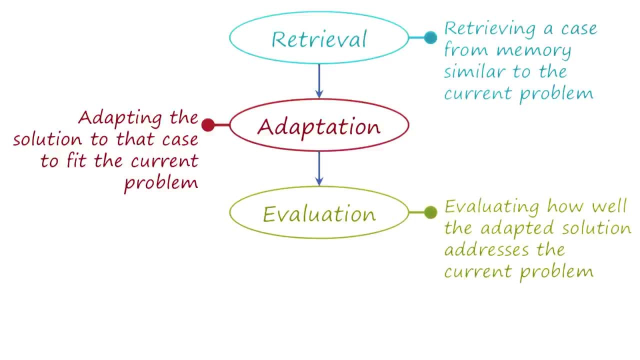 will have a long, такого-assimilated indication that's left empty or a similar cause. here, That is antiquated salvation in the two challenges of via backward and direct. fourth, When the user is able to come back, we'll be able to evaluate whether the solution actually succeeds in meeting. 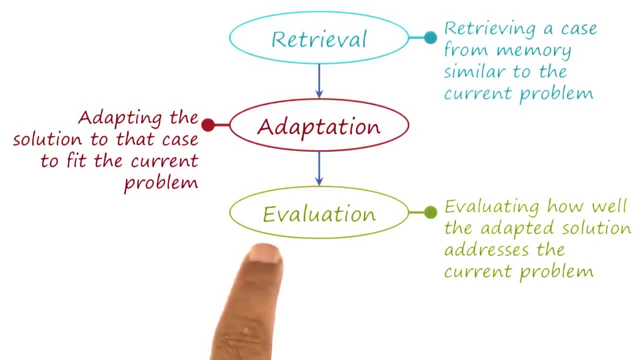 the requirements of the problem. For the programming problem, once we have a new program that we obtain by adopting the old program, we can actually run the program to see whether or not it will meet the requirements of the new problem. Let us suppose for a moment that we evaluate the candidate solution and 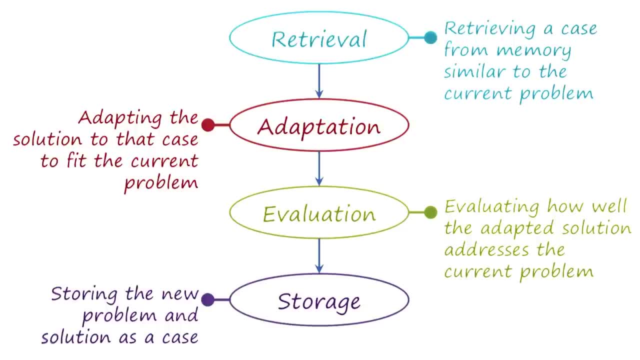 it succeeds, Then we could encapsulate the new problem and the new solution into a case and store it back into the case memory so that the case memory is constantly increasing. Notice that this case-based reasoning process unifies memory, reasoning and learning. There is a case memory that contains a large 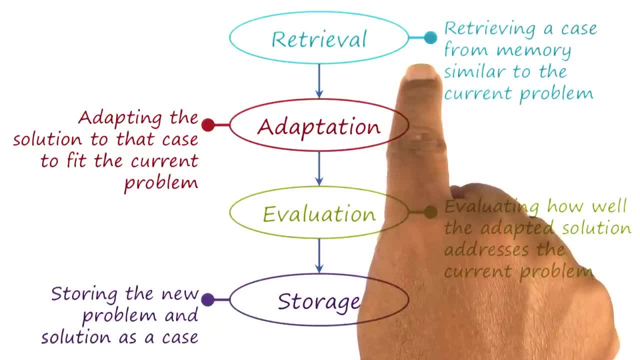 number of cases and that's how we retrieve cases that are relevant to the current problem. We'll reason when we adopt and evaluate and we'll learn when we store the new case back into the case memory.